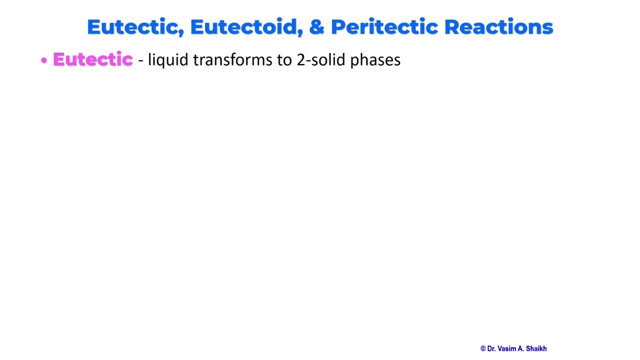 So now, what is eutectic reaction? In eutectic reaction, one liquid phase will transform into two solid phases. So one liquid phase will transform into two solid phases. So here, as an example, we will be looking at the lead and tin phase diagram. 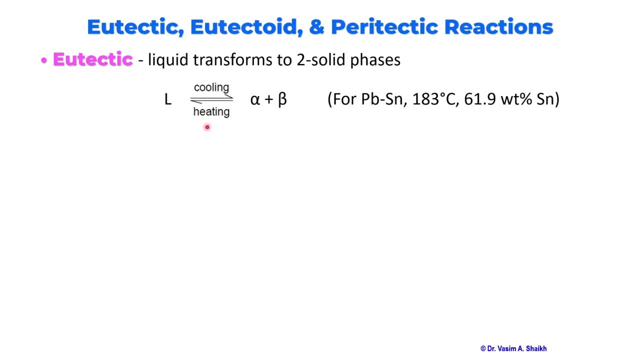 And you either heat or you cool. This is what you will be getting. So if you are here and having two phases and you are heating the material, then it will transform into liquid and when you are cooling the material, it will transform into two solid 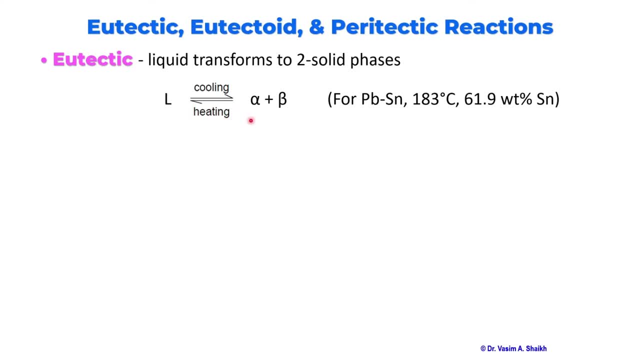 So liquid, one liquid phase will transform into two solid phases. That is called as a eutectic reaction. And these reactions- eutectic, eutectoid and peritectic reaction- all these reactions are invariant Means they will be happening at a particular temperature and at a particular composition. So that is the main thing here, which we have to remember in a particular phase diagram. 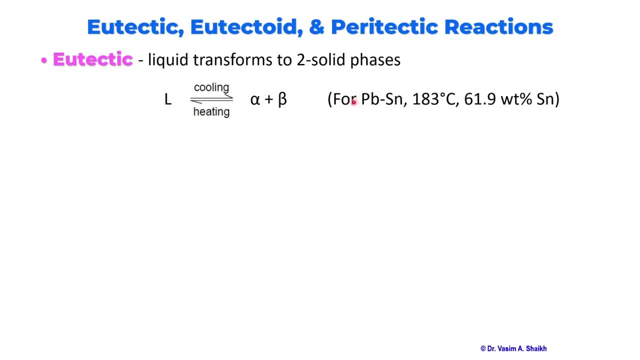 So here we are looking into the lead and tin phase diagram And here In the lead and tin phase diagram, at around 183 degree Celsius, at the composition of tin, we will be having this eutectic reaction. So in the upcoming slide we will see exactly the phase diagram and we will see the eutectic reaction. 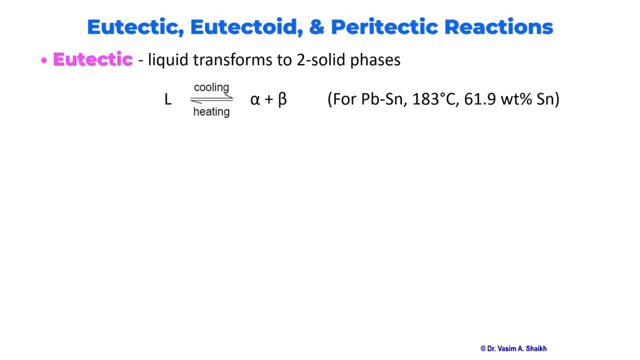 But before that we will be looking into all these three reactions, Then we will be looking into the phase diagram of these reactions. So next is eutectoid reaction, And a very common and very important Easy example for us to remember is from the iron and carbon phase diagram, where one solid phase will transform into two solid phases. 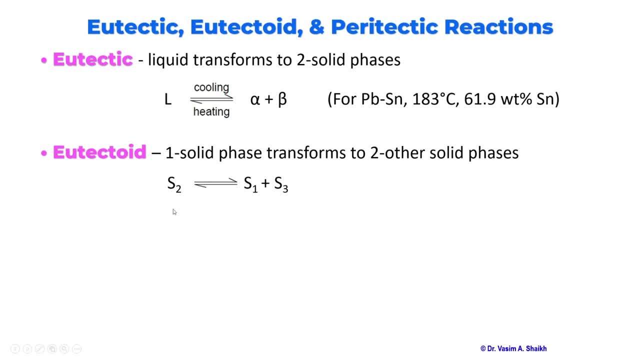 So, overall, one solid phase- here as an example, we will see S2, that is a solid phase- will transform into S1 and S3. And however we do it, we either heat or cool. we will get the same thing after heating and cooling. 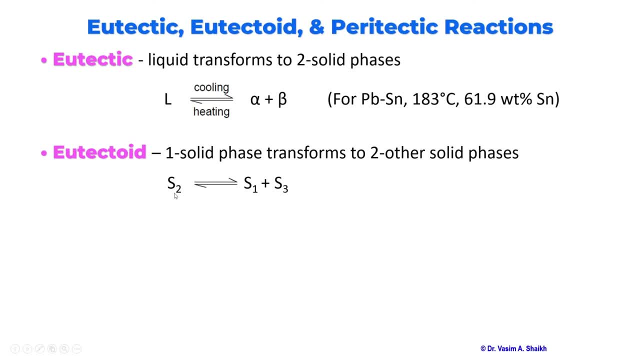 So when we are cooling from S2, we will get S3.. So when we are cooling from S2, we will get S3.. So when we are cooling from S2, we will get S1 and S3. 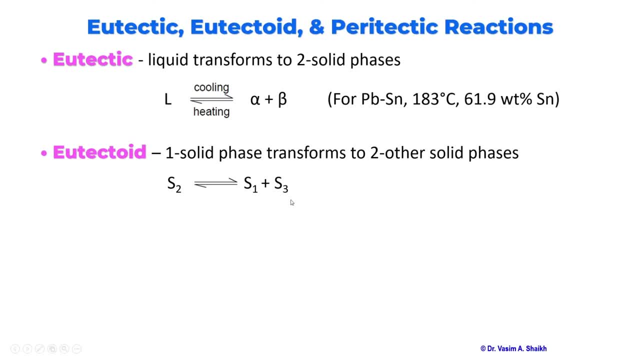 And when we are heating from S1 plus S3, that phase will give us one solid phase. As an example, we have earlier, earlier we have seen the iron carbon phase diagram. So at around 727 degrees Celsius, at the weight percent of 0.76 carbon, we have this particular eutectoid reaction. 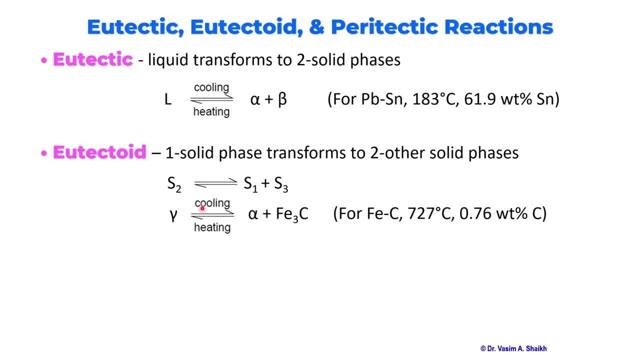 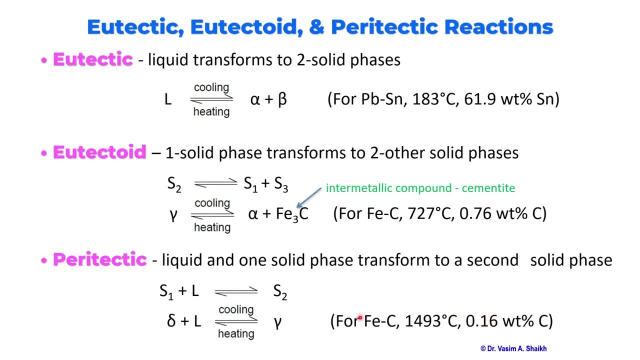 So gamma phase. when we are cooling the gamma phase we will be forming alpha phase: 0.16 weight percent of carbon delta, that is a solid phase, and liquid will transform into gamma, which is nothing but austenite phase. but again, in the upcoming slide we'll be not discussing about. 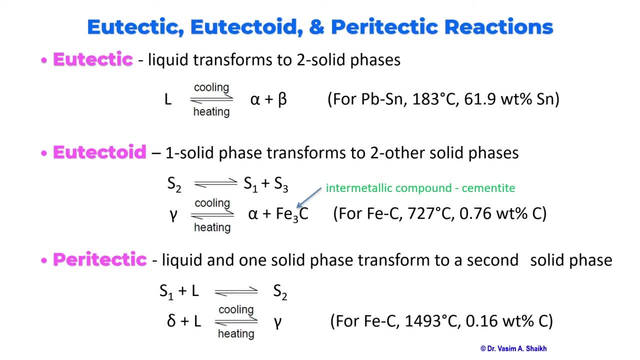 ion carbon phase diagram because, again, we have seen this transformation in that video. so we will be looking at a new phase diagram where we'll be studying about the peritectic reaction. so just remember that solid plus liquid will give us another solid. that is the peritectic reaction. 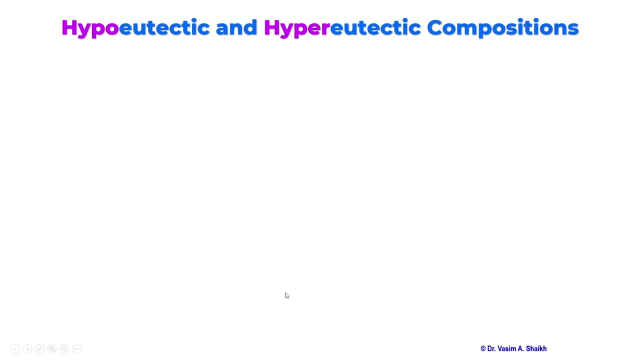 so now one more very important point here which we need to know, in the eutectic reaction or the eutectic compositions, that we have two eutectic compositions and these two compositions are hypoutectic and hyper eutectic. similarly, we can even have a hypoutectoid and 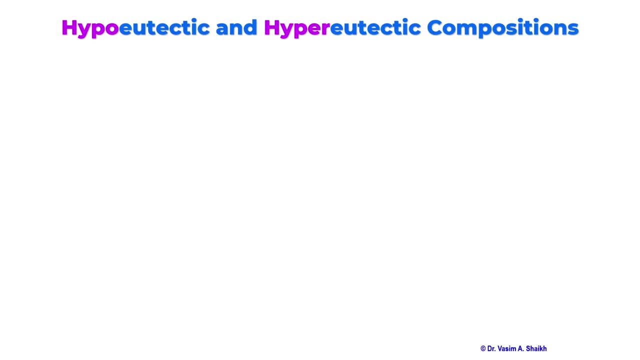 hyper eutectoid composition. now, what is this hypo and hyper eutectic composition? just, we'll just have a look at it. so this is the lead tin phase diagram, this is a lead tin phase diagram, and this composition here is the eutectic composition. this is a eutectic composition, as we have seen. 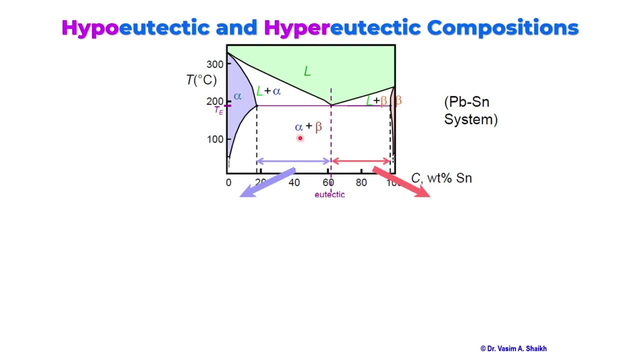 earlier, liquid will transform into two solid phases at this temperature, at this temperature and this composition which we have seen. so this is an invariant reaction which is not going to change. it will be same at this phase diagram. now, what is hypo eutectic? now hypo eutectic. 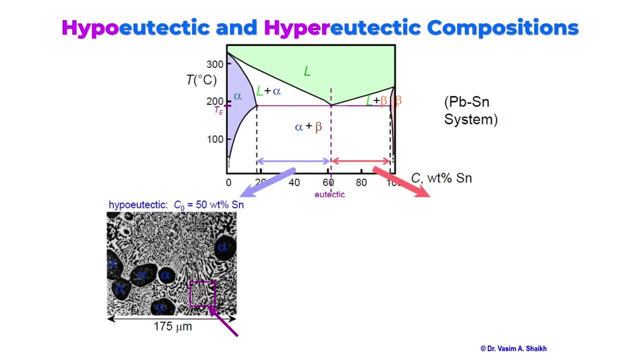 is nothing but the composition which is to the left of the eutectic point, or eutectic composition. so here, this area which is shown is the hypo eutectic composition. so this is the hypo eutectic composition, which is to the left of the eutectic point, and exactly at this particular composition we have 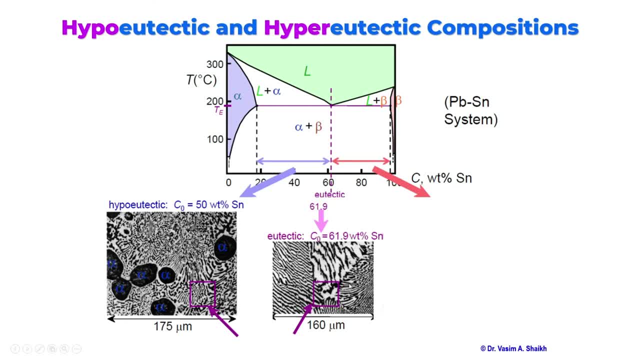 the eutectic point. so this is the, the microstructure or an actual image of the eutectic phase of the material, and this is the exact composition of hypo eutectic material and this is the actual image of the hypo eutectic alloy. similarly, we have 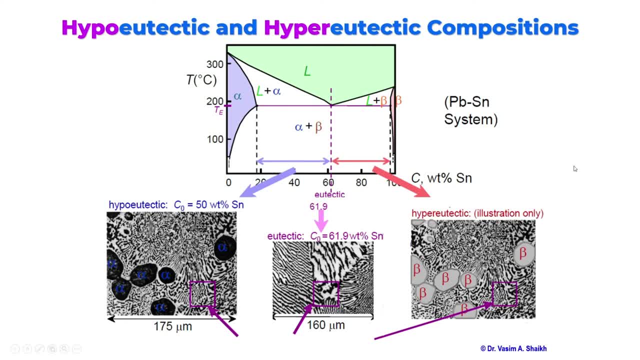 hyper eutectic composition and this is the hyper eutectic. so here you can see that when we are just below the eutectic point and from there there onward, if we draw a tie line it will hit the alpha. so all the hypo eutectic composition will have alpha. so this is the 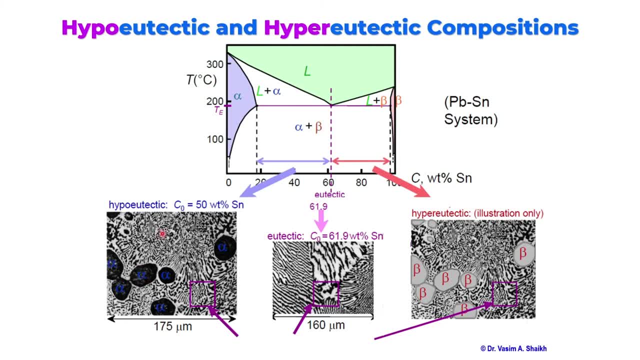 alpha which will be having and then rest will be the eutectic composition. now there is a particular name which is given to this particular alpha, which is called as a pro eutectic alpha. so pro eutectic means before the eutectic this alpha was present. so this is that same alpha. okay, so that is called. 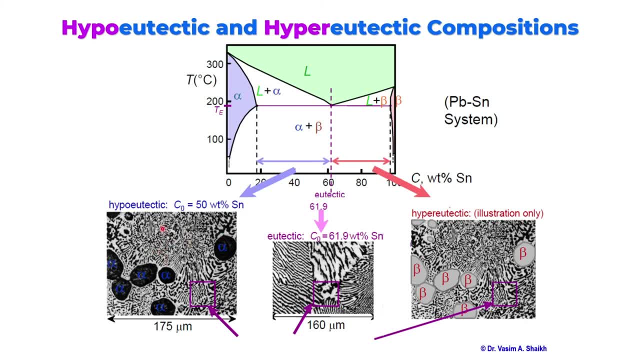 as a pro eutectic alpha and this is the eutectic composition. so the eutectic composition will consist of the lamellar layer, will consist of the lamellar layer of alpha and beta here. okay, so that is the eutectic composition. now hyper eutectic composition will have beta. will have beta because 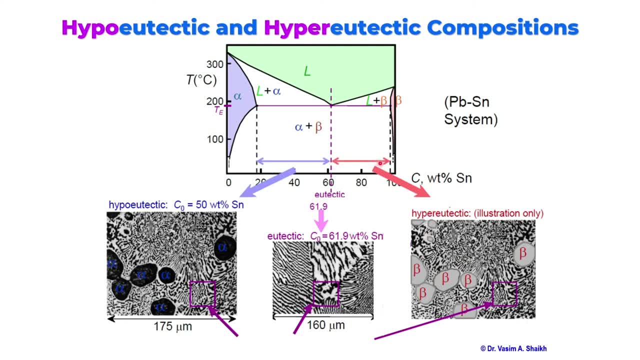 from here. if you draw the tie line- imagine this is a tie line, okay, just above this, you have the tie line and you draw the tie line, so that tie line will hit the beta, so it will have beta, okay, and it will have the eutectic composition. so beta and eutectic composition, and again one more name. 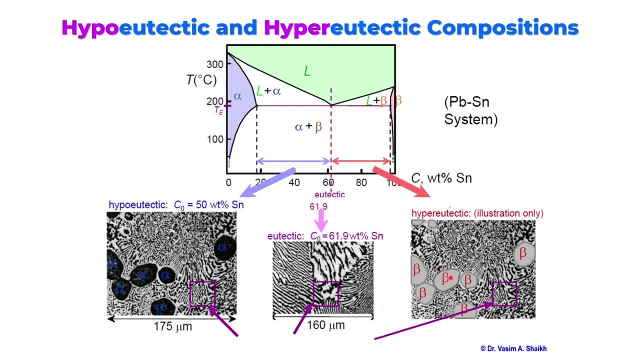 is given to this beta is that it is pro eutectic beta. okay, pro eutectic beta, so on. you know, in in whole, you know as a whole phase, beta is present and beta is also present in this alpha and beta eutectic composition. now, all these are: 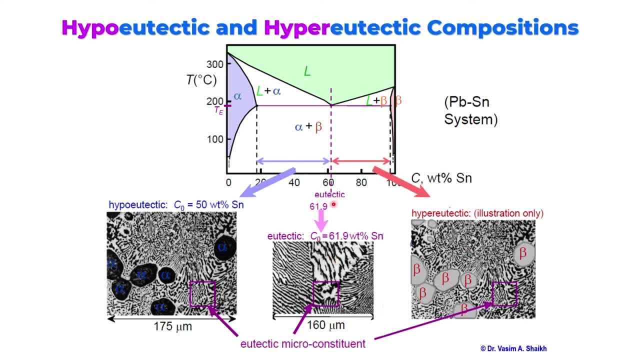 called as the eutectic micro constituent, because some eutectic is present in both hypo eutectic and hyper eutectic alloys, and the hyper eutectic composition will be to the right of the eutectic composition. so to the right of the eutectic composition, whatever the composition is there. 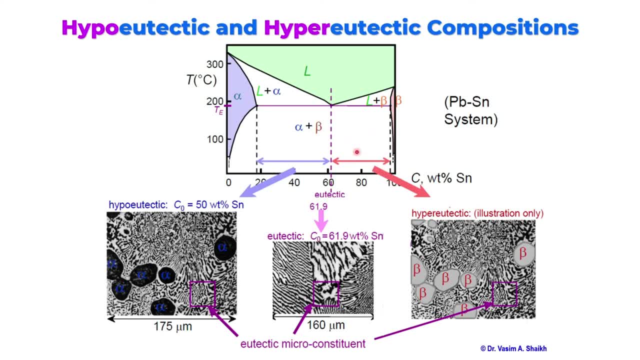 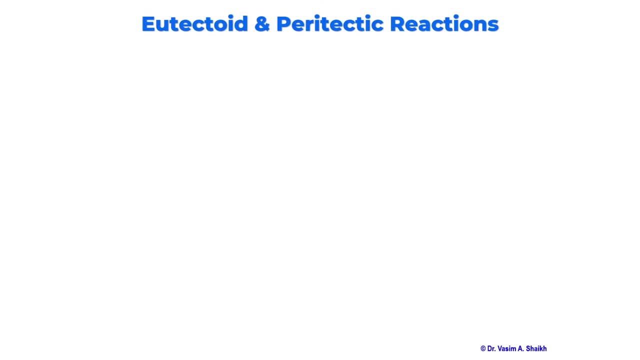 we call that as a hyper eutectic composition that i forgot to mention earlier. now coming to the second and third reaction. so we have seen eutectic reaction and hypo and hyper eutectic reactions, or the composition we can say, and now we will look into eutectoid and peritectic. 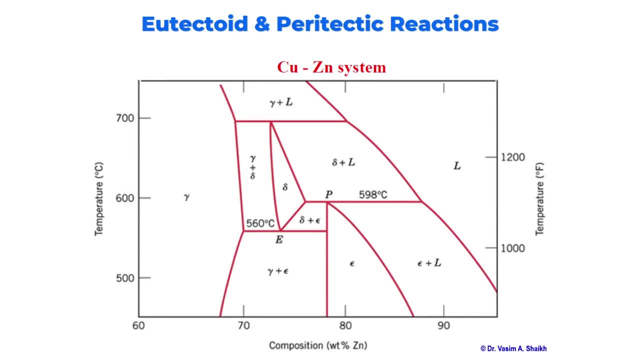 reaction. now, what is eutectoid and peritectic reaction? let us have a look based on this copion and zinc system. so this is a copper and zinc phase diagram. now let us look into the eutectoid and peritectic reactions here. so looking into the phase diagram. 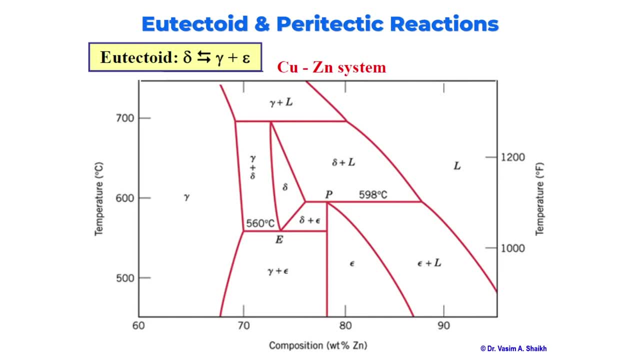 here we have a eutectoid composition. so, as we have seen in the earlier slide, eutectoid is nothing but one solid is transforming into two solid phases. so your Delta is transforming into gamma plus epsilon. so you can see here: this point E, this point E, this is a delta phase here. okay, and exactly at this. 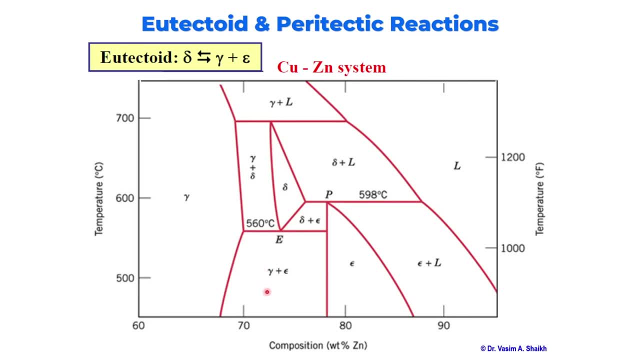 point E, just below that, it is transforming into two solid phases, two solid phases. so this is temperature on the y-axis and composition on the x axis. weight percent of zinc is on the x axis and exactly at this point one solid, that is Delta, is transforming into two solid phases. that is